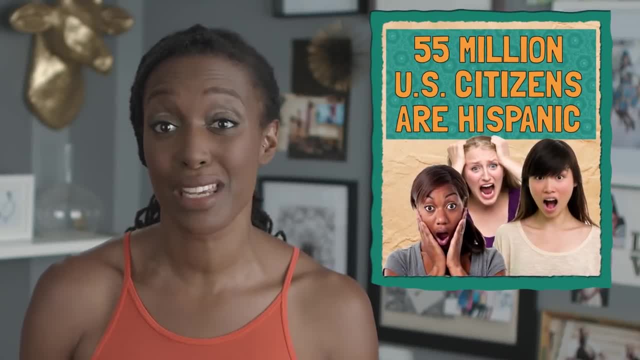 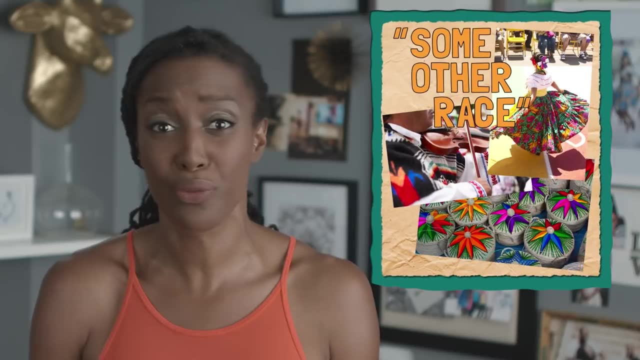 Not only is this a hell of a shock when you consider that over 55 million US citizens are Hispanic, but I guess the some other race category is supposed to be a passive-aggressive catch-all for their beautifully diverse culture, And even that option doesn't really work. 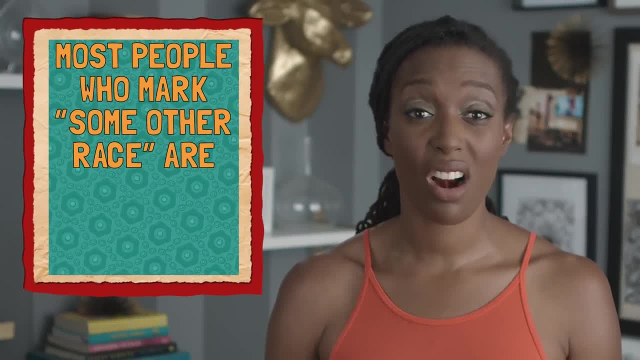 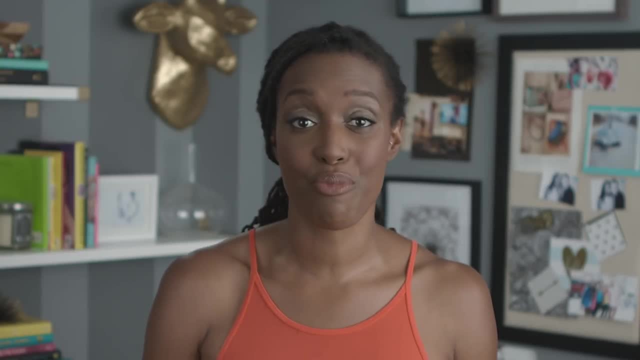 In the US Census Bureau, most people who mark some other race are often counted as white. So if Hispanic isn't a race, then what is it? Well, before we get to that, we actually have to settle another important thing. 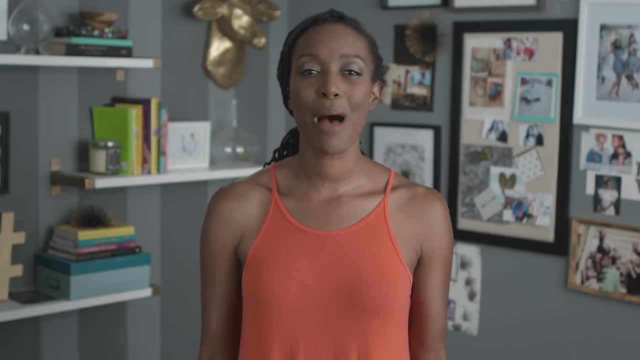 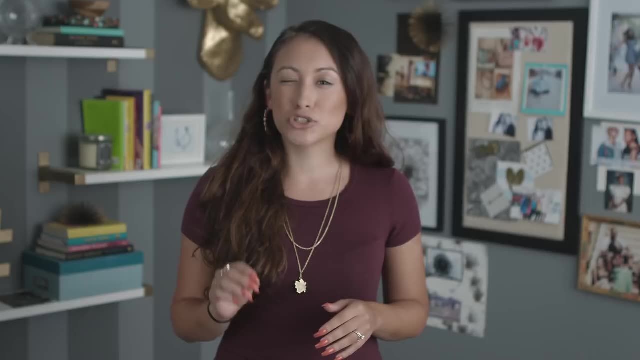 What's the difference between Hispanic and Latino. So I'm gonna enlist some help from my friend, Kat Lazo. Thanks for having me, Francesca. So it may get a little confusing if this is your first time hearing this, so I'll try to keep it as simple as I can. 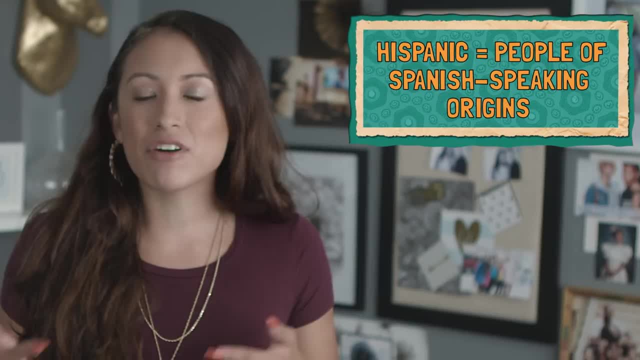 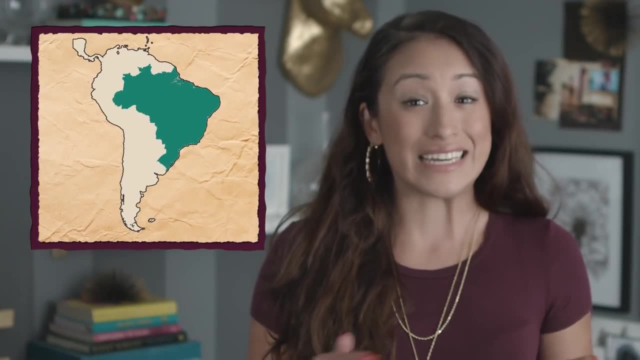 Hispanic refers to people of Spanish-speaking origin. It means you have a family history in a Spanish-speaking country. This means you have origins in these countries, including Spain. But notice how Brazil isn't included in the map. Well, that's because they don't primarily speak Spanish. 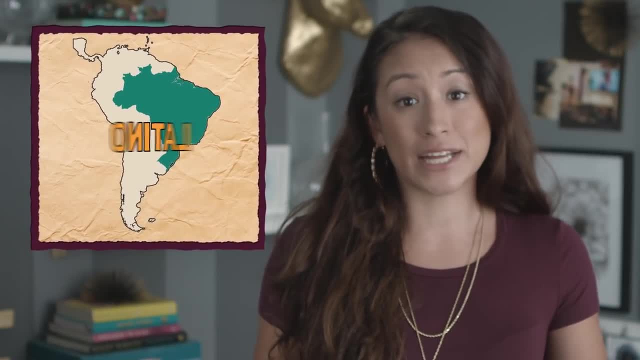 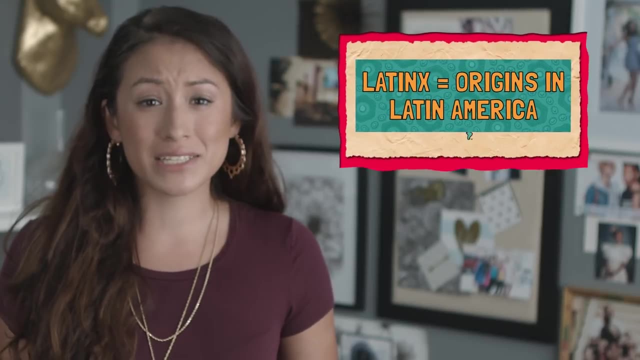 They speak Portuguese, which brings us to Latino, or Latinx, if you wanna be gender-inclusive, which you should be. Latinx refers to having origins in Latin America, which is basically the countries in North and South America that are geographically south of the United States. 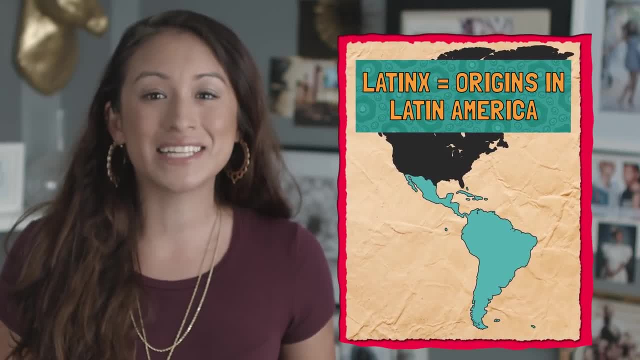 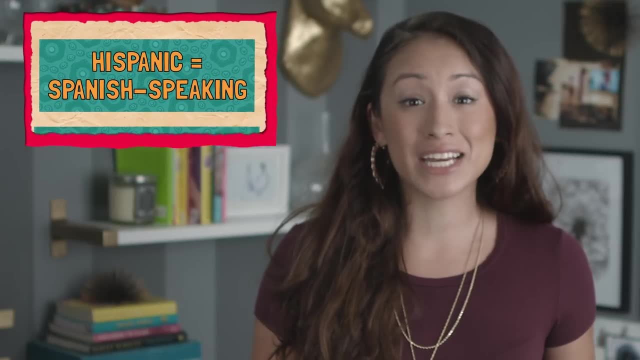 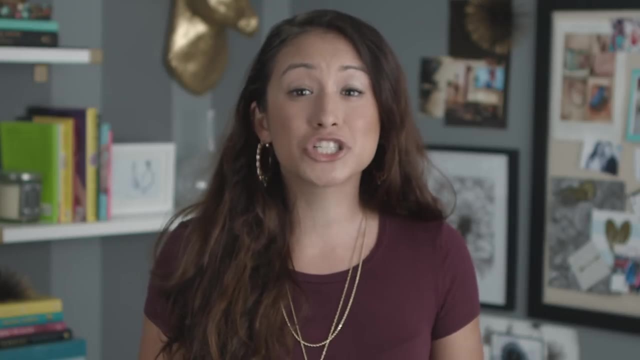 including most of the Caribbean And, unlike Hispanic, Latinx excludes Latin America's colonizer, Spain. So one more time, Hispanic refers to language and Latinx focuses on geographic location. But whichever term you use, neither of them actually refer to racial identity. 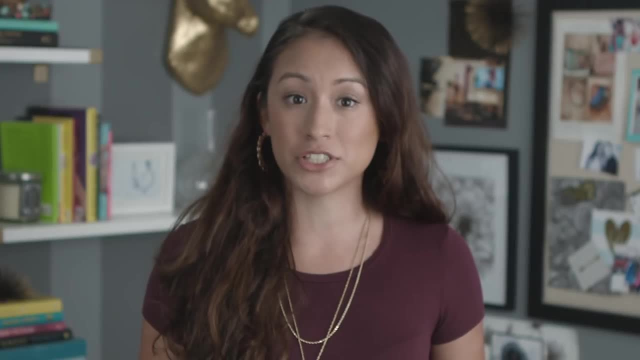 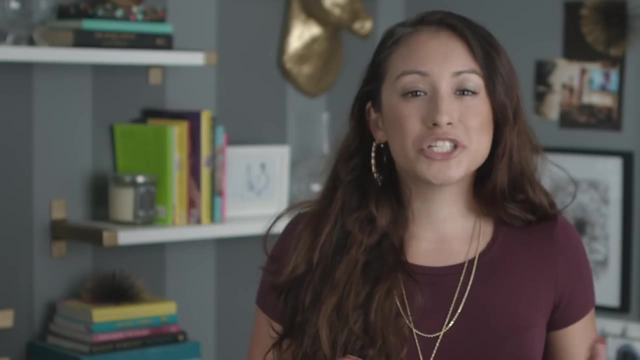 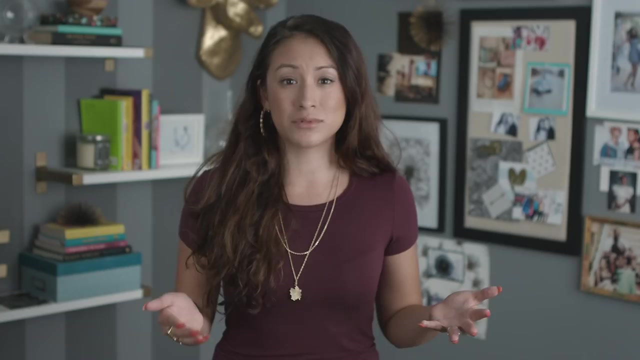 Just like America, Latin America has a long and complex history that intersects between native people, European colonization, African slavery and global immigration patterns, which is why there are white Latinos, native Latinos, black Latinos, Asian Latinos and every kind of mixture that you can think of. 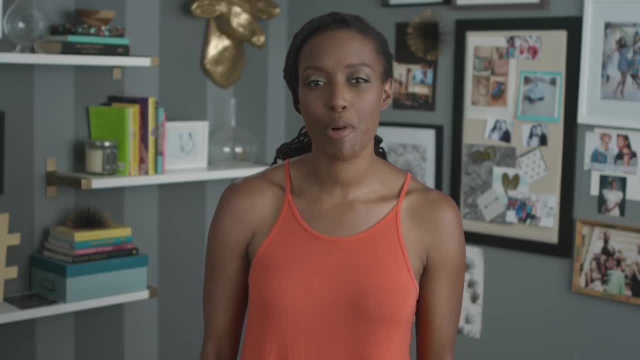 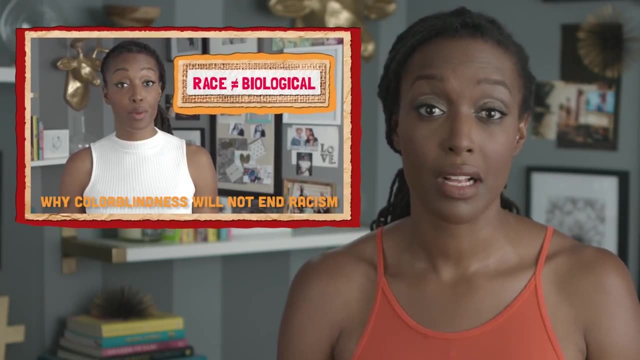 Does that help? Yeah, that does help, But I think part of the problem we're dealing with here is the broader confusion between ethnicity and race. As we've covered, race is not biologically real. It's basically an ever-shifting categorization. 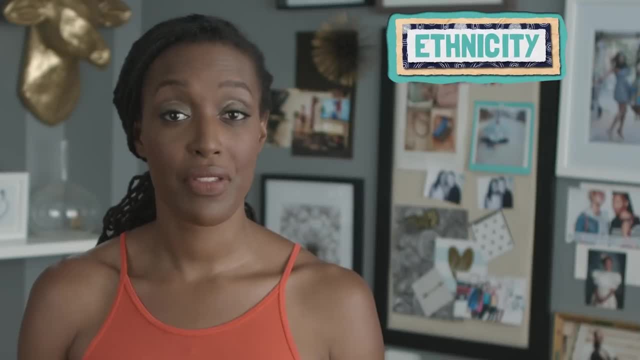 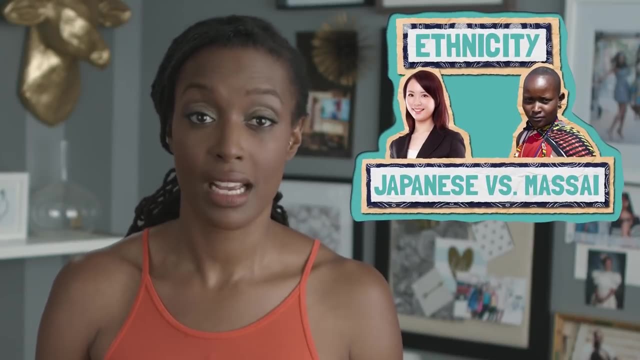 that sometimes includes ethnicity and sometimes doesn't, But when it comes to ethnicity, there are legitimate differences between groups of people that aren't based on external characteristics. And, yes, ethnicity can get fuzzy, but there are cultural practices you can associate with it. 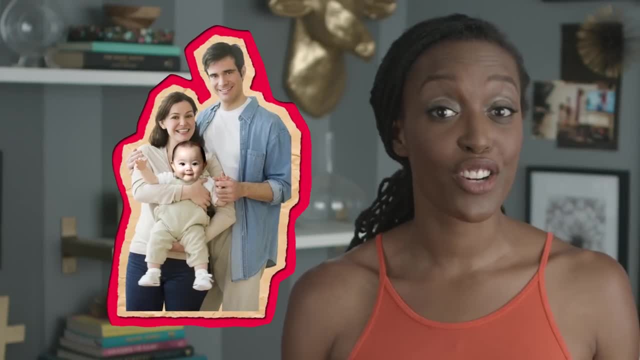 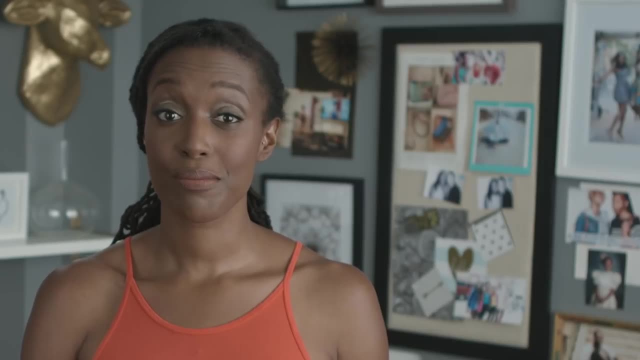 like language, cultural values and traditions, which is why, if an Argentinian couple adopts a baby from China, that baby will most likely grow up speaking Spanish and rooting for Lionel Messi. The simple answer: Race doesn't exist, but ethnicity does. 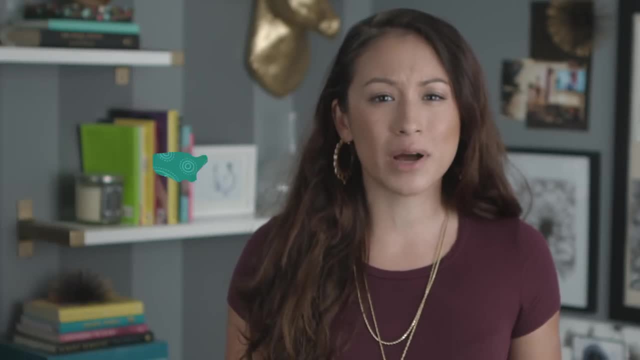 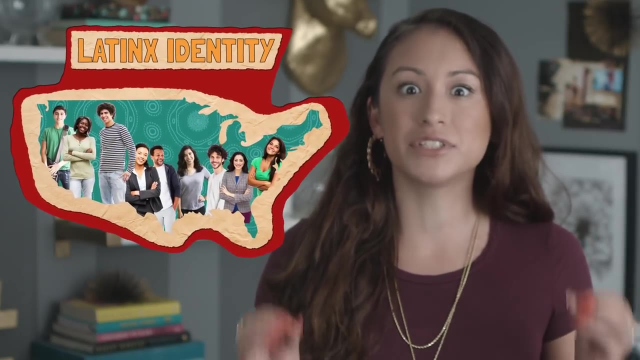 Exactly The reason this gets so confusing when we're talking about Latinx in America is that there's a broad ethnic Latinx identity that has a complex history, with lots of different racial groups living together. Latinx isn't a race, but we're definitely racialized as a people. 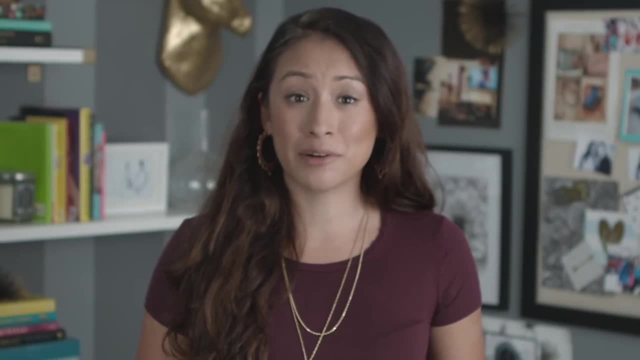 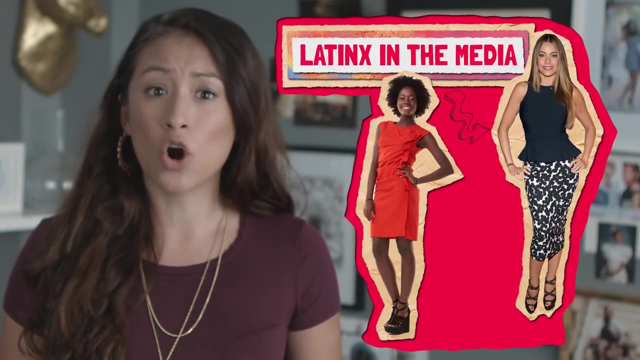 which is confusing, and I'm the one who said it. The US and Latin American media has done a great job at constructing an image of what Latinx look like, and that image is rarely black or fully indigenous, for example. We like the rest of the world. 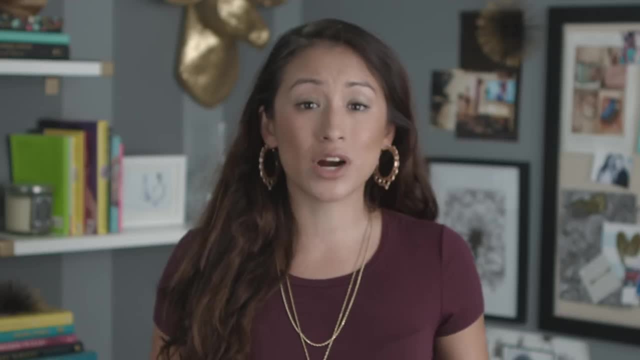 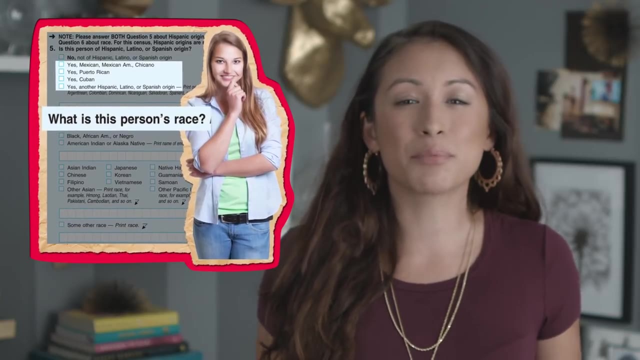 have internalized these messages of white supremacy through the media and through our education. So it's no wonder that when Latinx here in the US are confronted with deciding their race based on the census in a predominantly black and white binary society, many of us default to white. 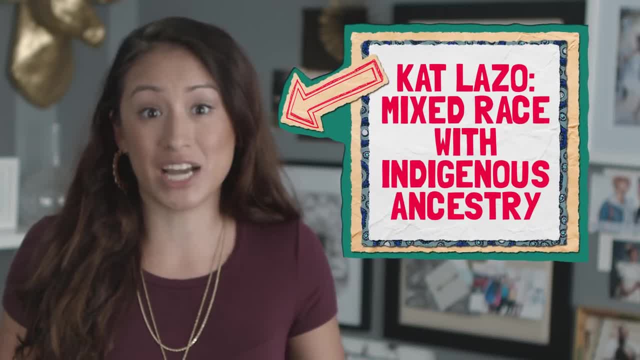 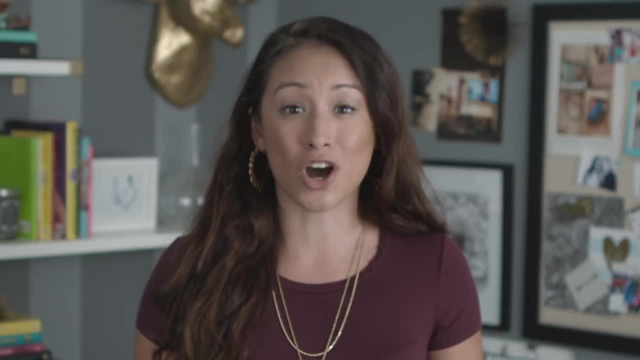 I personally identify as a mixed-race Latina with indigenous ancestry, but that's just me. There are a multitude of ways that Latinx choose to identify racially, but it's up to us to unlearn much of what we've been taught about race. 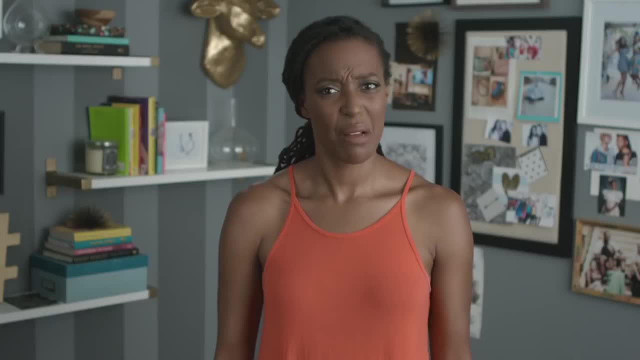 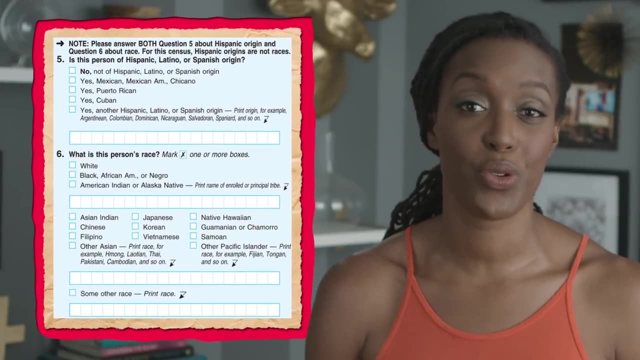 and demand better and more accurate forms of representation. Damn, there has to be a better way to talk about this. Well, there is a better way. The census is planning to make changes in 2020 in one huge way. They're going to stop using the word race altogether. 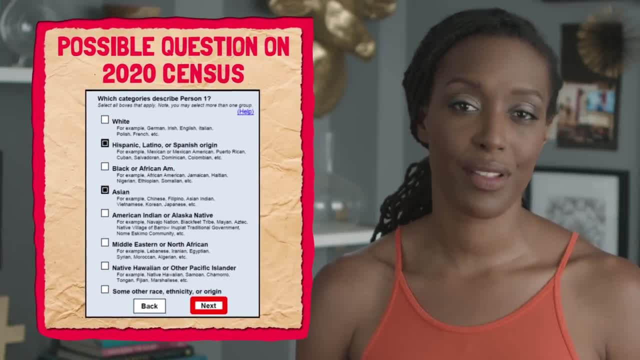 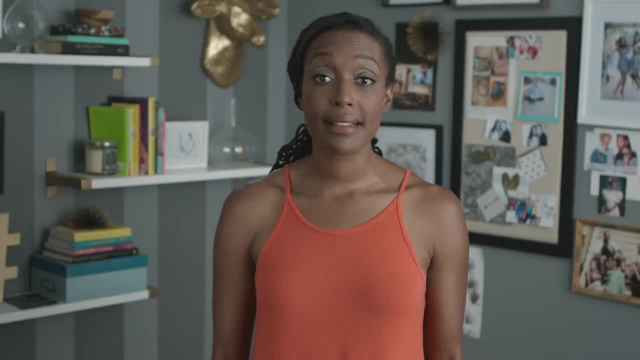 Hispanic, Latino and Spanish origin will be a category like everything else, with no qualifiers. That means people will now check the categories that best describe them. This will not only give us a better idea of how many people identify as Hispanic or Latino. 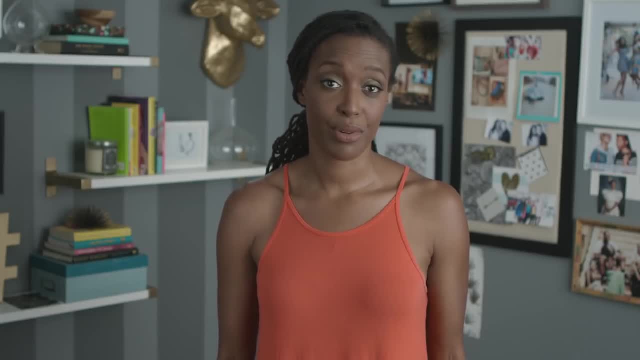 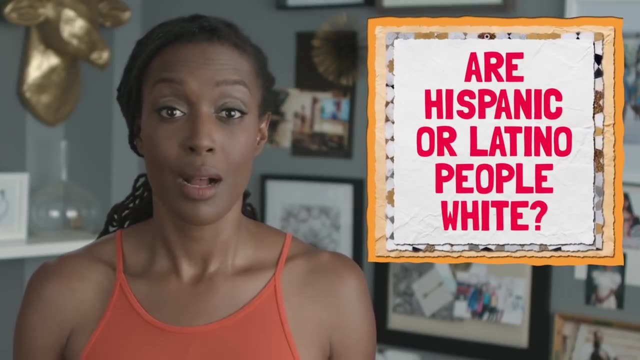 but could also give us a better idea of multiracial and multiethnic numbers. So to return to the original question: are Hispanic or Latino people white? Well, some are and some aren't, But to quote the 2013 Census Bureau report: 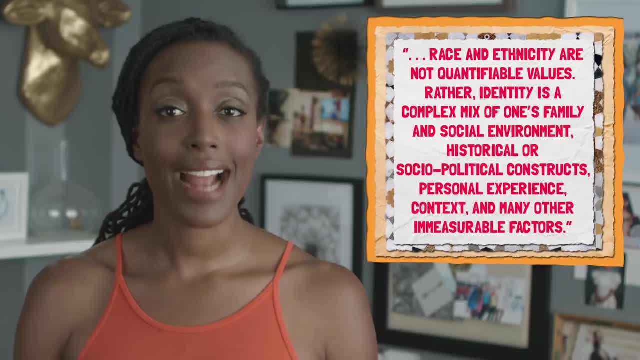 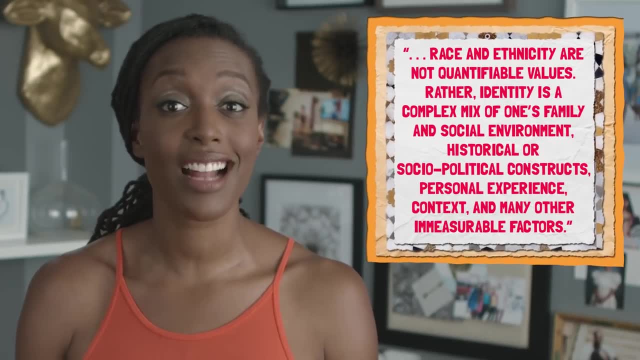 race and ethnicity are not quantifiable values. Rather, identity is a complex mix of one's family and social environment, historical or sociopolitical constructs, personal experience, context and many other immeasurable factors. Hmm, surprisingly woke coming from the census.